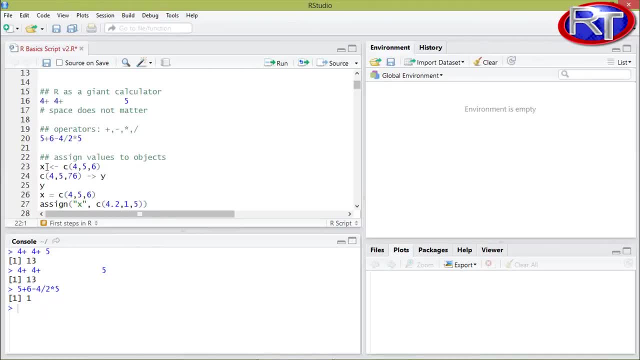 Therefore, we have several ways of how we can create objects and we have several ways in how we can do assignments. So the first one would be: we can use this kind of arrow sign, which consists of the smaller sign and the minus sign, The arrow. 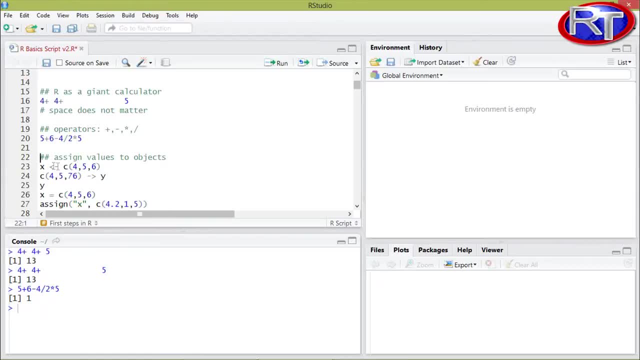 It always points towards the name of the object. So in this case I call the object x and the arrow points to this side. In this case, I'm calling the object y and the arrow points towards the y letter. When you have a collection of numbers or values, you would have to use the concatenate function. 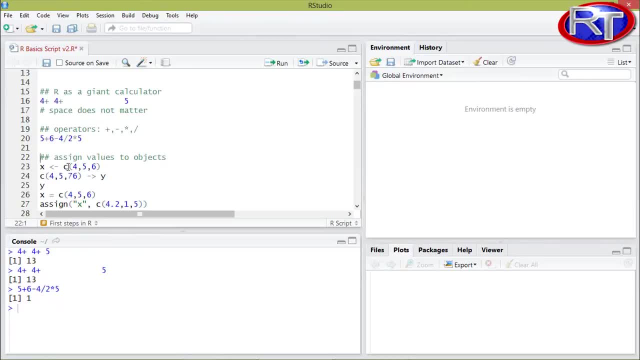 to somehow bind all those values So concatenate, or c is a really, really important symbol, And you should keep that in mind. So let's run this line to exemplify what happens if you do that. Alright, so now you see that you did not really get an output. 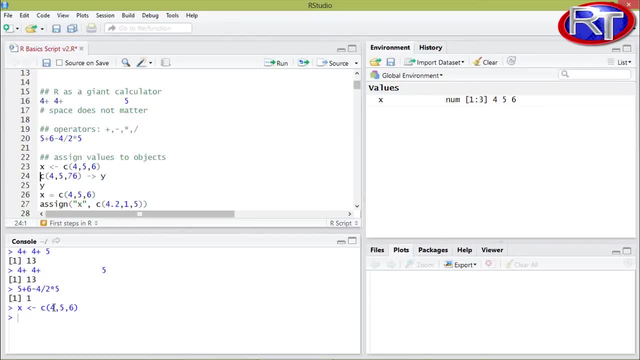 You only see in the console that this script line was actually executed. There is an important thing that happened to the whole RStudio program. now Over here in the global environment you can see that there is a new object For this value x And there is also some sort of information. what is inside this object? 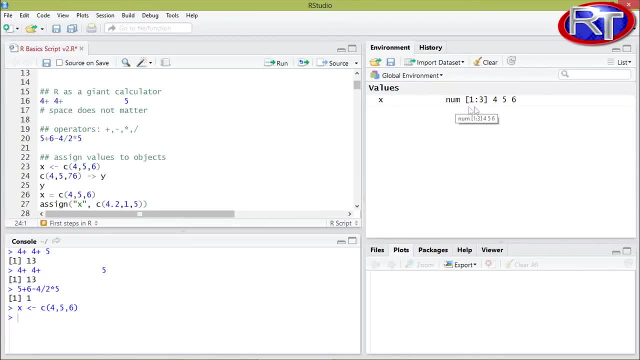 In this case, we see that it is a numerical object with three values, And then we also see those values over here, which are four, five and six. So this was basically the first object we created in R And, as you can see in this line, 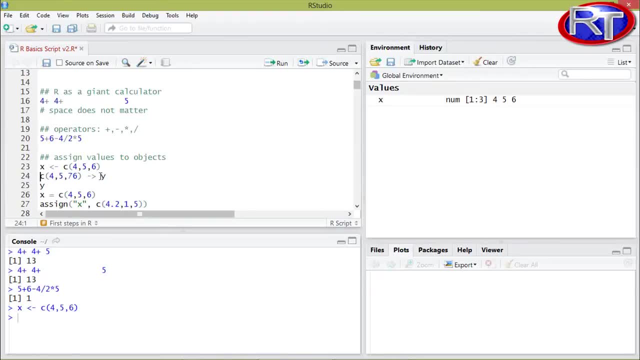 down here We have the same setup, But now the name of the object is at the right side and the arrow points towards this symbol, again Towards the y. So again we have another object, The object y. If we want to send this whole object now to the console and we want to see some more in, 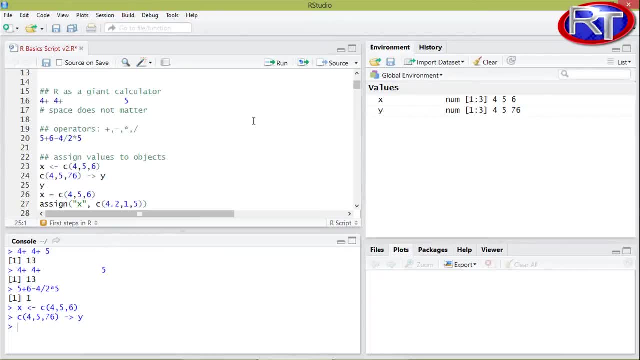 depth information about this object. We can just type in the object name, which in this case is y, And we could run this line. As you can see, We have the output also in the console. Another way in how you can create object and how you can do assignments is simply by using 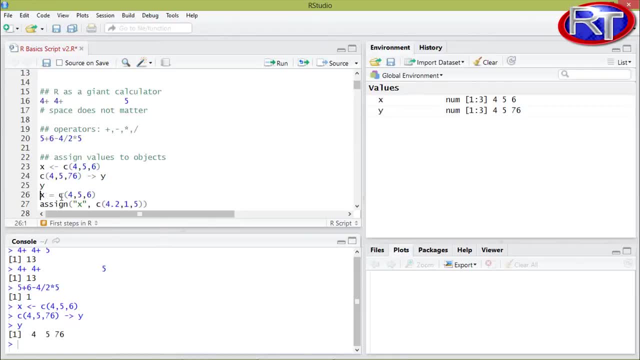 the equal sign. So in this case x equals concatenate and have the numbers four, five and six as my example numbers, And this would basically do the same thing as we did in this line over here. We again created the object And now we have the output. 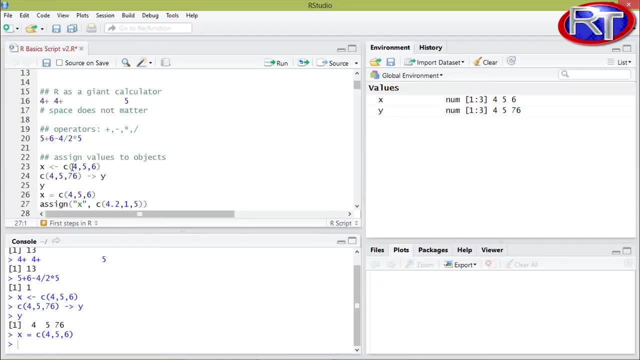 The object x. Another way in how you can create objects and how you can do assignments is by using the assign function. By using this function you would then in brackets- normal around brackets- You would state the name of the object under quotation signs And after a comma you can again use the concatenate function and insert the values which should. 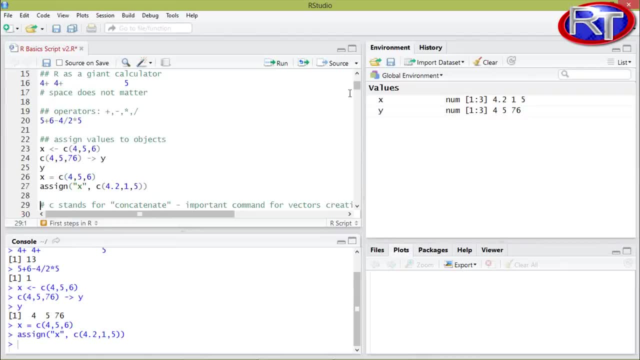 be inserted in that vector. And By running this one, you now see that the object x has changed to these numbers up here which we specified within this concatenate function. So those are the ways in how you can create objects and how you can do assignments. 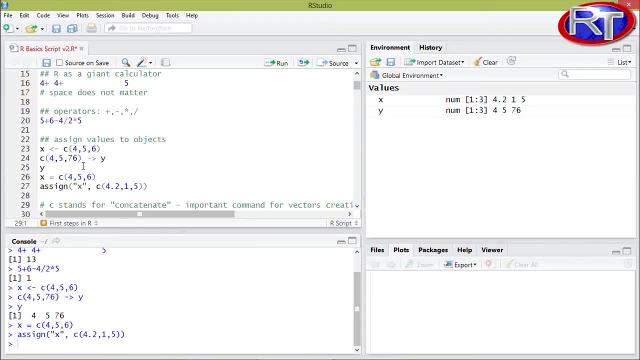 And you will see those things in many manuscripts. So this is a crucial and very basic feature of R: To actually see or to learn which objects we already created. We can use the assignment function, We can use the ls function, So it's ls and empty brackets. 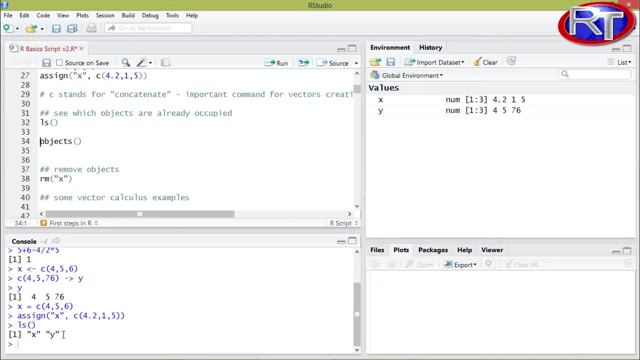 And if I would run this line, you would now see in the console which objects are already created or which object names are already occupied. The same thing would be by using the objects command. So again, objects, empty brackets. If I would run this one, I would get the same result. 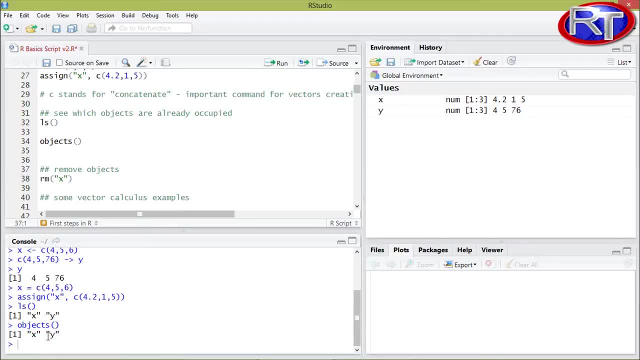 And basically the output In those lines Down here should be the same as you see in the global environment. So it is basically all about those values or those object names which you can also see in the global environment. If you actually want to remove the object, you can use the RM function. 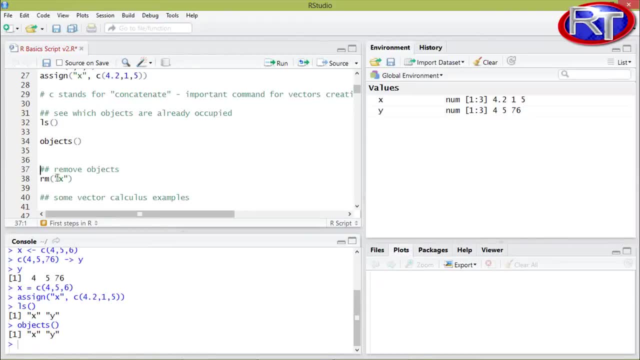 So in this case it is RM, brackets, quotation signs, and then the name of the object which you want to remove. In this case it is the object x. So if I'm running This one, You now see that in the global environment we do not have the object x anymore. 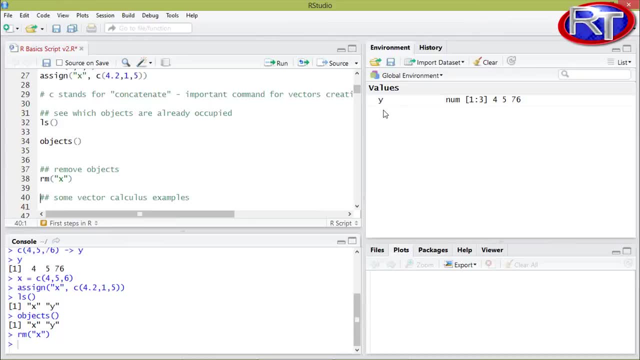 Please note that in case you already have the object x in your environment but you are creating a new object with the same name x, the old object would simply be overwritten. So then you would lose the old object x. Let's take a look at some vector calculations. 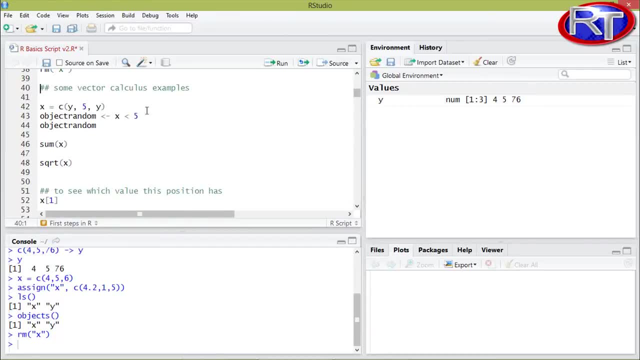 So what you could do is you could create another vector or another object by using already existing objects. So in this case, I'm creating the object x by using the number five and two times the object y. So let's take a look at this line and, as you can see, now we have seven elements within. 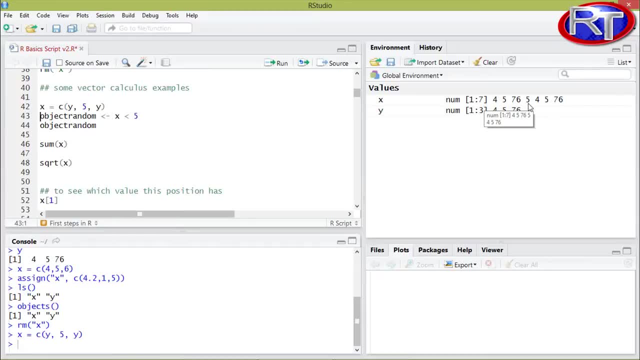 this object and the middle element is the number five and those other two elements are four, five and seventy six, which is the object y. If we actually create the object random, which actually shows us which elements of the object x are smaller than five, we would get this output down here: 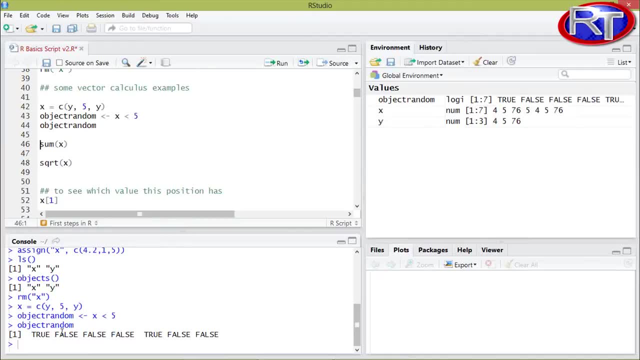 So this is a new vector. It's the object random and this is a logical vector containing only true or false values, and those values show us On which position within this object random, this criterion over here is met. So all those places where x is smaller than five should be marked as true, and all those 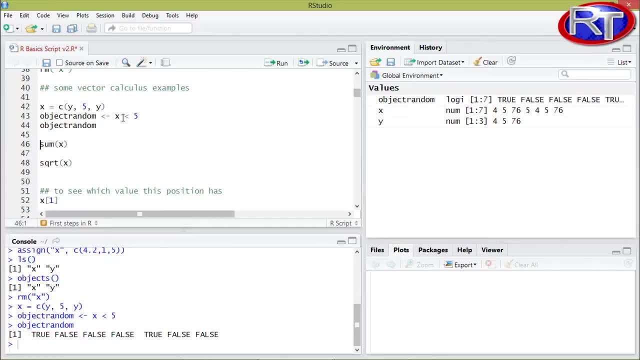 positions where this criteria is not met should be marked with false. So let's take a look at it. We know that x looks like this, and now we should actually take a look on which positions those values are smaller than five, Because on those positions we should have a true as an output, and this is basically. 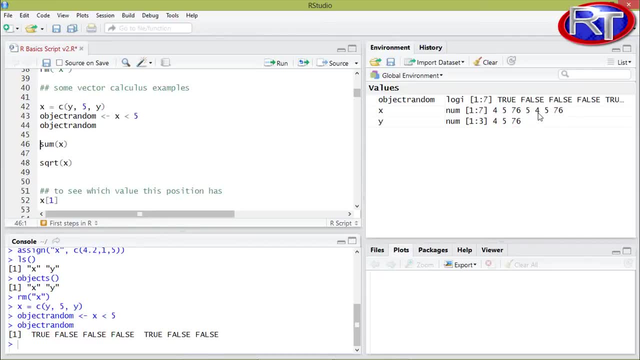 on this position is the first position and this position, which is the fifth position, and, as you can see, we have a true on the first position and a true on the fifth position. So this is actually how a logical vector looks like. We can do, of course, some kind of other calculations. 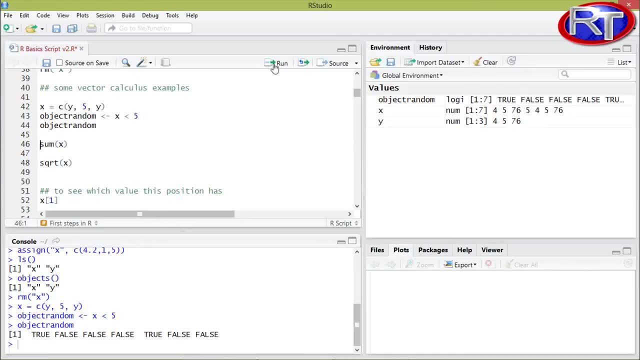 We can get the sum of our object x If we would run this one. all those numbers in this vector are summed up and this gives us the value of hundred and seventy five. as you can see down here, We could also get the square root of every value within the object x. 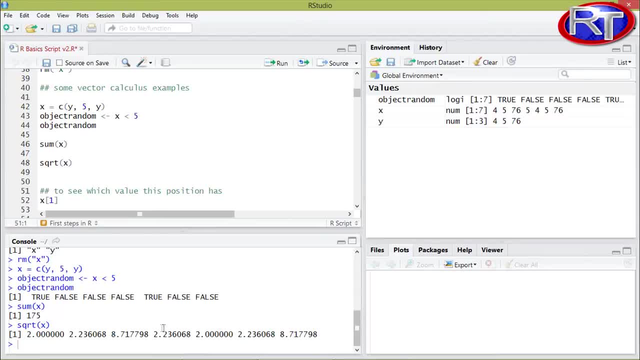 If we would run this one, the output looks like this: So, for example, the square root of four is two, and this is what we get over here. The next thing we could do is We could take a look at our object x and we can see which value we've got on position. 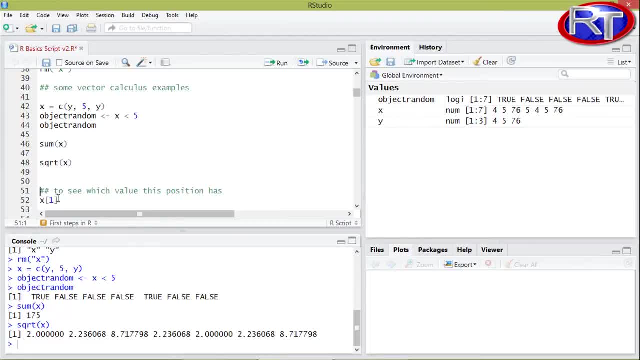 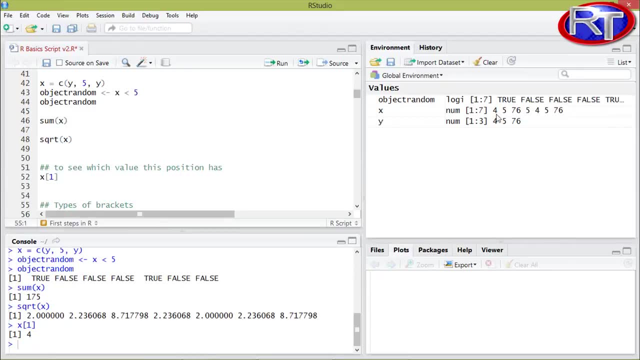 number one. So please note that those box brackets are always about index positions, So let's run this one. So basically, what this should show us now: it should give us the output four, because four is on the first position within this vector, and of course we have the output four. 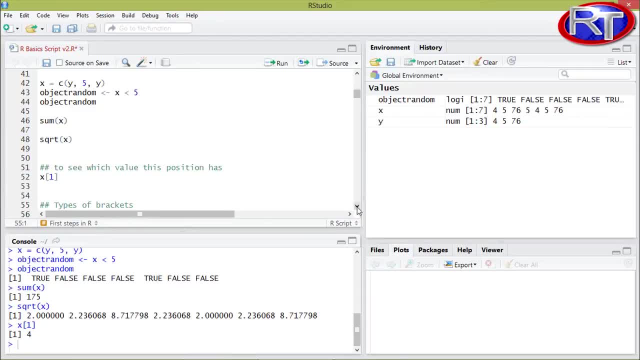 down here. The last thing. The last thing I want to show you in this video is that there are actually three different types of brackets. We have the round or normal brackets. We have box brackets and we have those kind of curled brackets. The round brackets are actually used for all those standard operations. 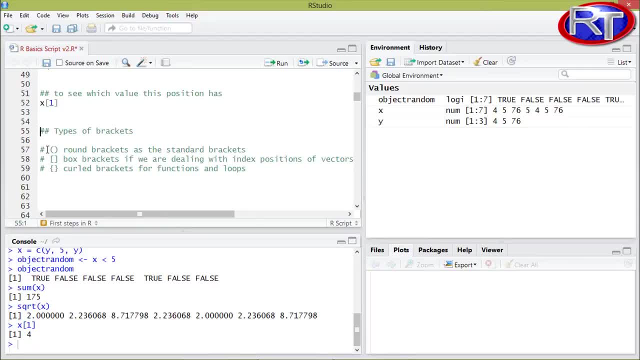 So, for example, if we want to create new objects or if we want to bind together several values, it's the round brackets to be used. Box brackets are normally used to specify index positions or to see which values are at which position within a vector. That's exactly what we did in this exercise over here.